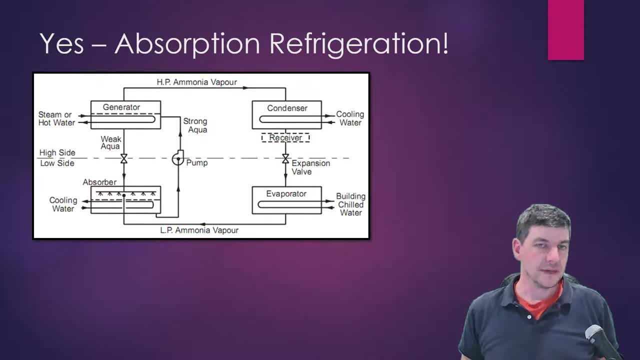 for a compressor and save a little bit on the energy side. Okay, the compressor is very good because it makes our cycle very simple And unfortunately, the absorption refrigeration cycle becomes a little more complex. Okay, and so this exercise. I'm going to walk through all the 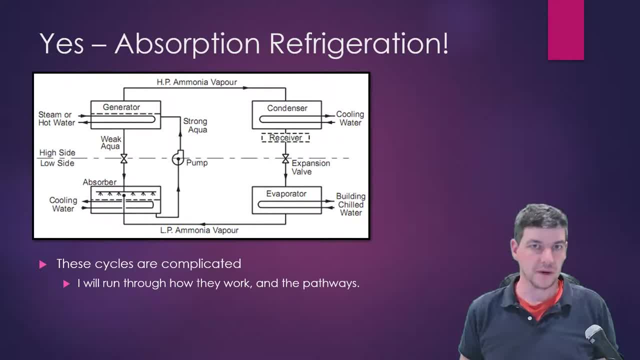 different cycles And I'm going to kind of explain to you how they different work. how they work and some of the terminology. I think it's handy if you follow along with me. So I'm going to be drawing some diagrams. I have some templates and you can either download them off of Blackboard. 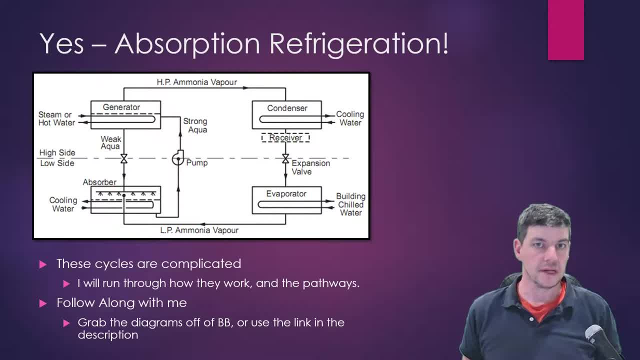 if you're using or you're part of the course, or else if you're just joining us on YouTube. I've got a link down in the description and you could download the template if you like, print it out and draw along with me. maybe helpful to you, Okay, so let's get started on our templates. 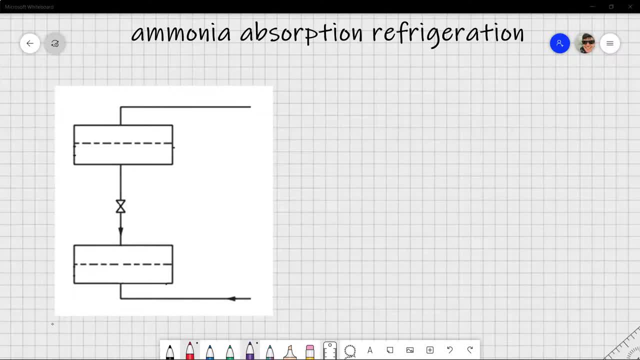 Okay, so the first system that we're gonna look at is known as an ammonia absorption refrigeration system, And we've used monia, or we've looked at ammonia before, and we know that it's typically used in industrial applications that need very cold temperatures. So we use it to make ice in a hockey rink, we use it for freezing. 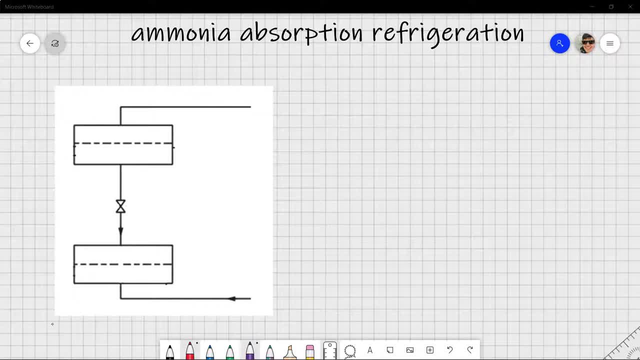 food. so this is something that we would use in that type of application where we have a need for very cold temperatures, So minus 30 degrees might be an example. Okay, so we're gonna sketch out this cycle and kind of understand how it. 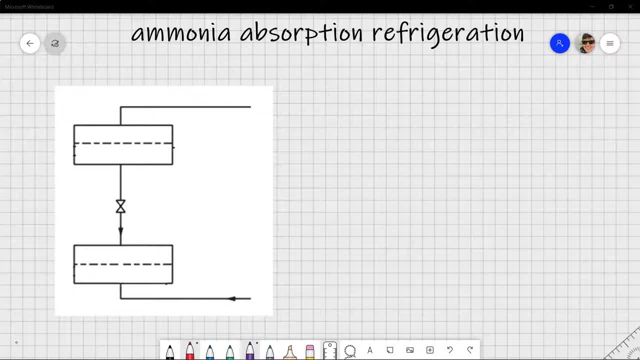 might work. Okay so, the first place that we're gonna start is in the vessel up here in the top. Okay so, this vessel here, and this vessel is known as the generator. Okay so, this is a generator and the generator. what it generates for us is ammonia vapor. 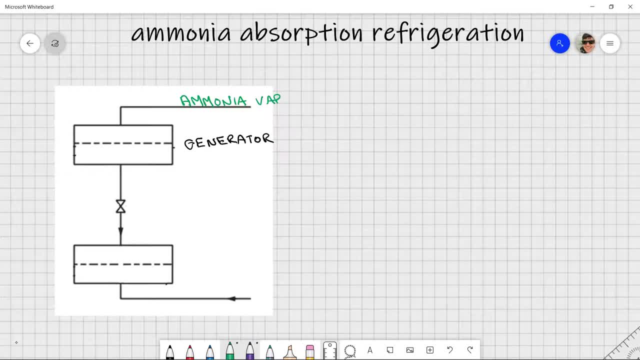 Okay, and how it creates vapor is inside of the vessel. what I have is a mixture of water and ammonia. Okay, so this is ammonia that's dissolved in the water. so I have a solution of ammonia and water, And what I'm gonna do is I'm gonna add a little bit of heat to it. Okay, so I've got some. 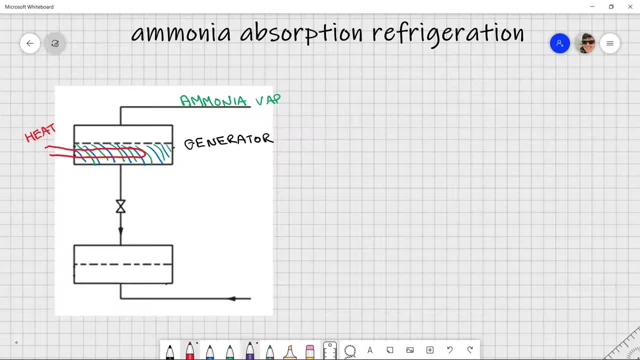 heat, and I'll need to supply heat to this cycle. And when I supply heat to it, what happens is some of my vapor starts to come out of the water Okay, and it's able to make its way into the racking area. I know a lot of oil plants have this. 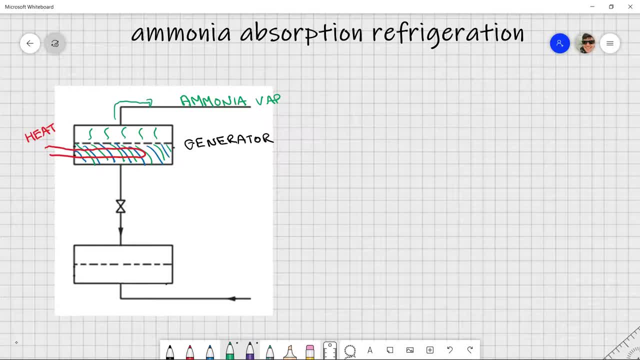 into the rest of the cycle. So I collect it and it's able to move on. Okay, so my generator has created some ammonia for me And that ammonia is then supplied to a more conventional refrigeration cycle. Okay, so we know, in a typical mechanical refrigeration cycle, after we've created some 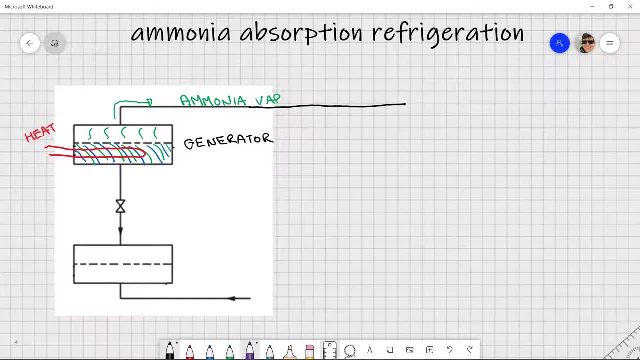 ammonia vapor and it's essentially at a high temperature or high-ish temperature because of the heat that's been added. where it goes to next would be a condenser, And my vapor is going to be turned into a liquid in the condenser And I would need you know some. 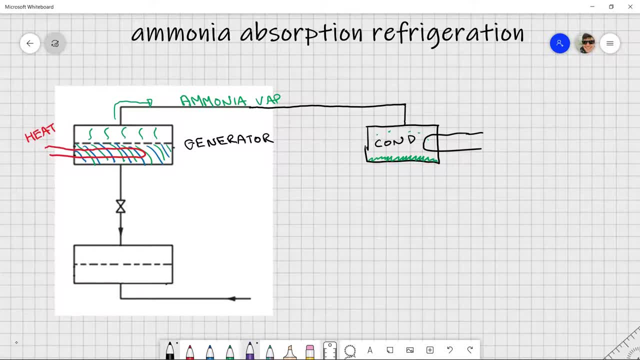 some cooling water or some heat transfer In and out of the condenser, Right, so we know we need some heat that's going to leave the condenser. It's then going to go to a metering device And then from there we go to our evaporator. 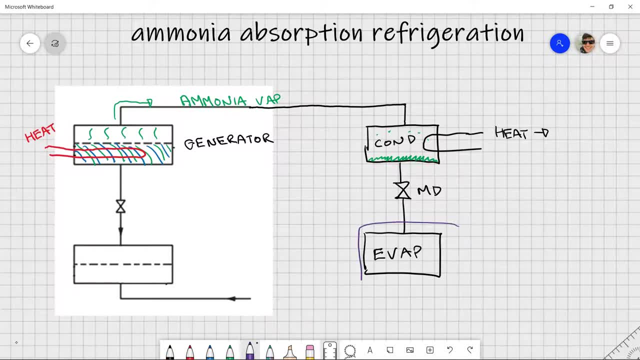 And our evaporator is typically going to be cooling a refrigerated space And you know that might be a typical application of ammonia. So, as I said, you know, maybe negative 30 degrees celsius or something like that might be the. 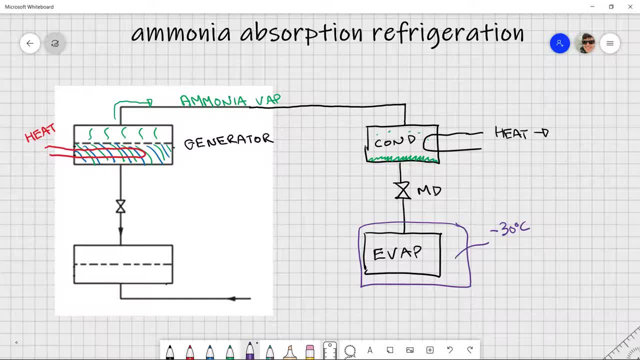 the bottom limit, So how cold it might possibly get inside of that cycle. From there, what leaves the evaporator goes back and revisits that components that I that I was talking about earlier And what leaves the evaporator, of course, is going to be. 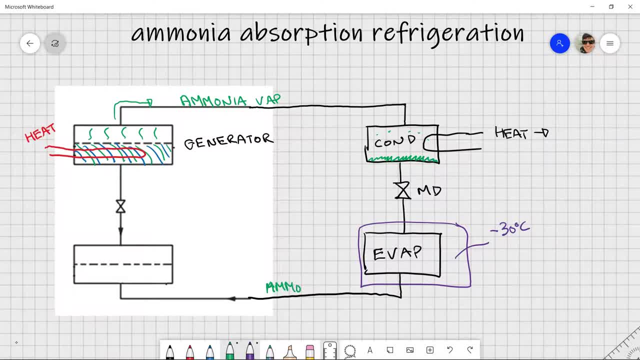 that amounts of ammonia vapor, Ammonia vapor, again This time at a lower temperature and generally lower pressure. that's going to make its way back. So The cycle as it runs right now, I would produce ammonia until my generator Started to run out of ammonia. 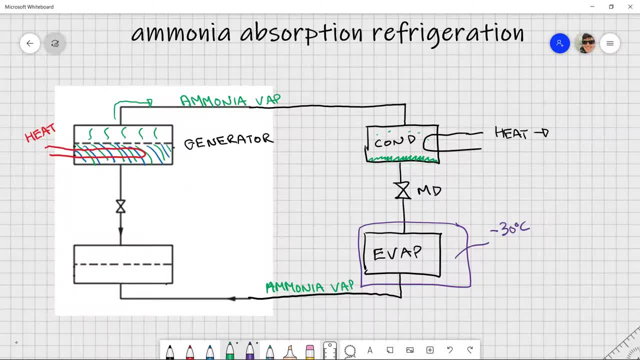 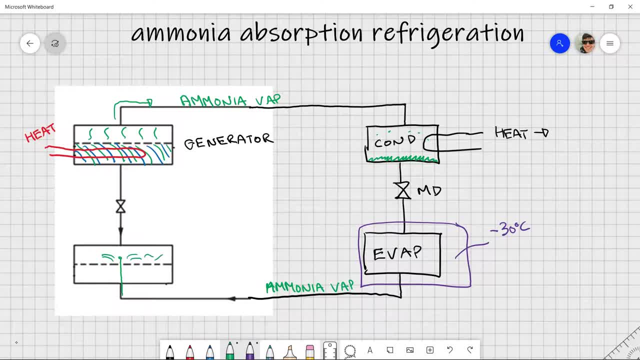 and sort of sort of make its way into this upper cavity. this vessel is known as the absorber, and we can imagine by the name what its function is. its function is to absorb that ammonia into something, and what that something is is going to be water. okay, here's where we get the water from: when we drive off the. 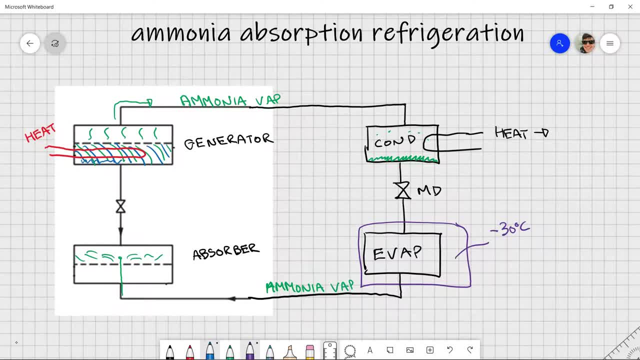 ammonia out of the jet. we get the water from when we drive off the ammonia out of the jet generator. what's left is mostly water. so we recycle that water downwards okay, and we put it into the absorber. now, generally, what we want to do is spray it. 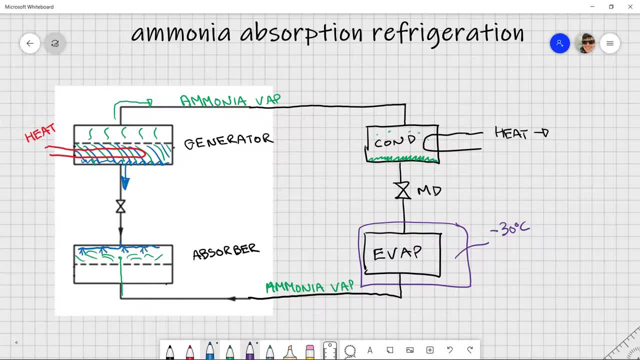 in so it can mix with the ammonia vapor that's in there and absorb it at the most efficient manner, and then what we're left with is down at the bottom. we've got now ammonia that's mixed with a water solution, okay, and so we now have lots of ammonia that's in that solution, and we 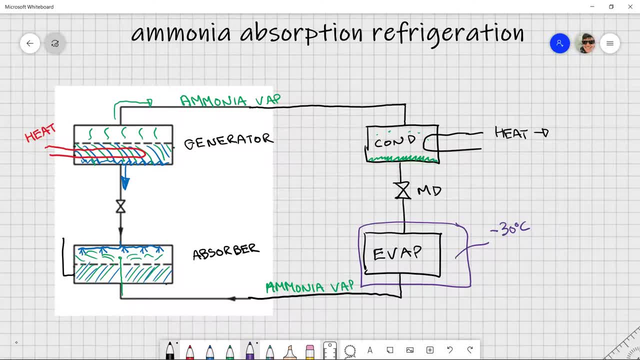 would take a little pump and we would pump it up and add it into, and we would pump it up and add it into my upper vessel. so we have sort of this circulation of water and when it's down at the bottom in the absorber it's absorbing ammonia vapor and becoming a 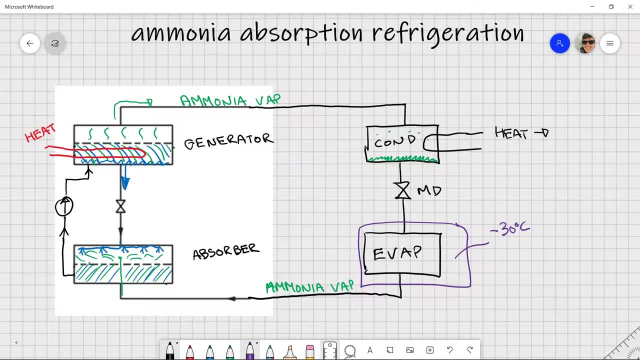 more concentrated ammonia mixture and then it's pumping it up to the top where we drive off some of the ammonia by adding heat and that creates a weaker water mixture and so we have some terms for the, for the those water mixtures. so up at the very top we have our lowest concentration of ammonia, so we have our 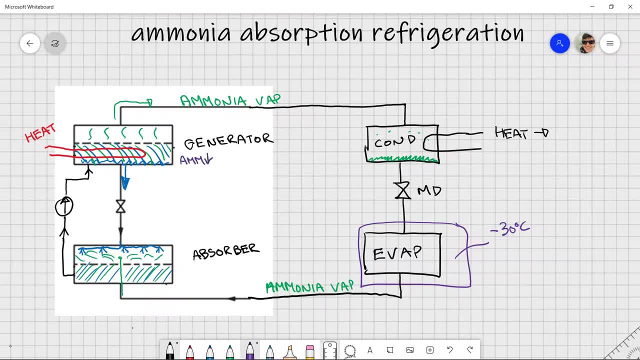 ammonia here, which is essentially a low concentration of ammonia, and that's what we would consider to be a weak solution and we call that a weak aqua solution. and down at the bottom here in the absorber, where we have a higher concentration of ammonia, we would 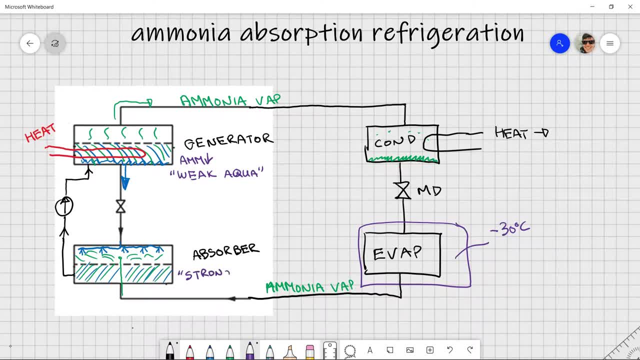 consider that to be a strong aqua solution. okay, so some terms. so we have four new terms. we have our generator, we have our absorber and we have our weak aqua and our strong aqua. the whole goal of this side of my cycle is to replace the compressor with 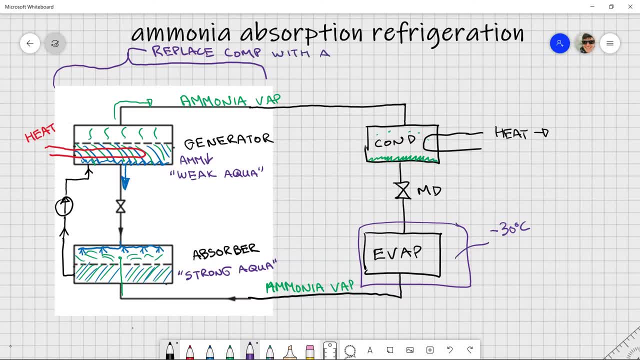 a pump and some heat. okay, so we think of the role of the compressor. it increases the pressure and it increases the temperature. in my cycle, here, in the absorption refrigeration cycle, what I've done is I have done those two things: increasing the pressure, increasing the temperature.